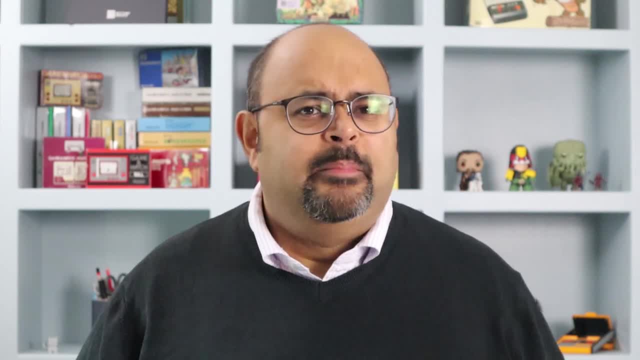 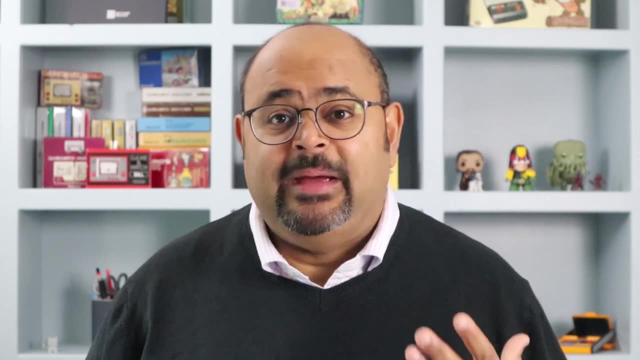 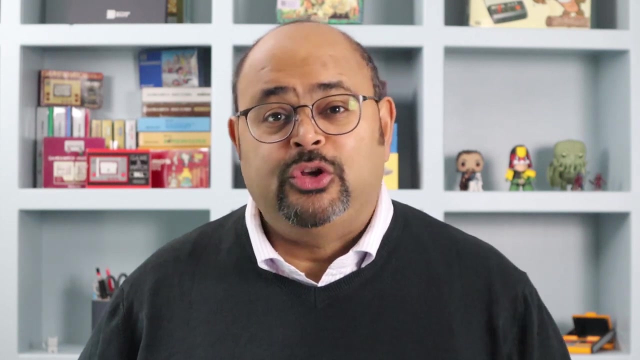 A game is a series of interesting decisions, But the board gamers of Reddit say that interesting just isn't enough. It's agreed that a good game lets you make choices, but those choices have to have impact to the game. A game should reward good play and punish bad play. 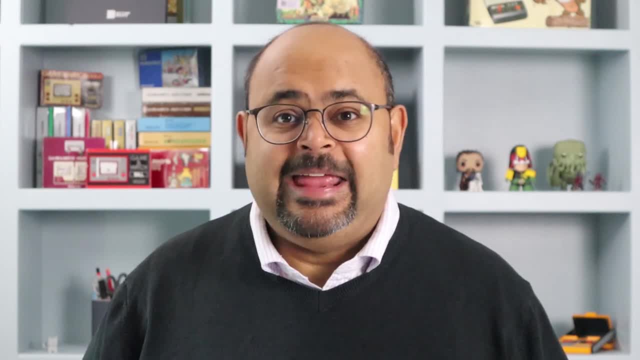 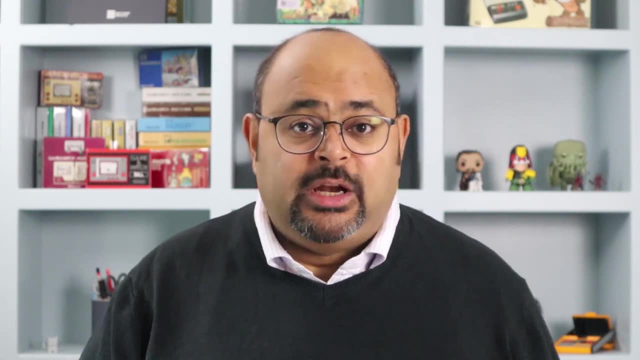 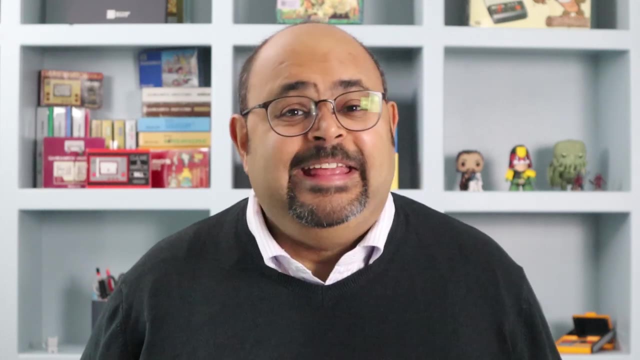 For a game to be truly good, what you do during play has to affect the outcome. Now, those choices could be Immediate, like choosing an appropriate clue word in a game like Codenames, Or they could be quite far reaching, like, well, almost any action in Race for the Galaxy. 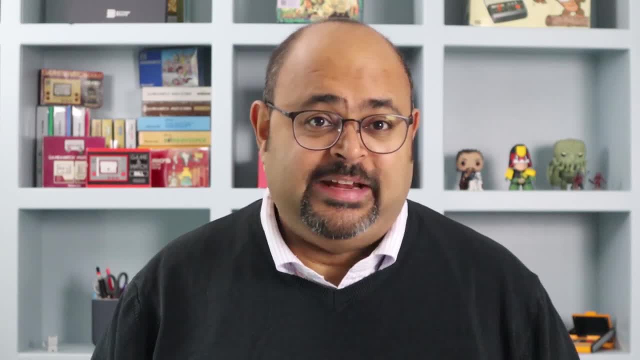 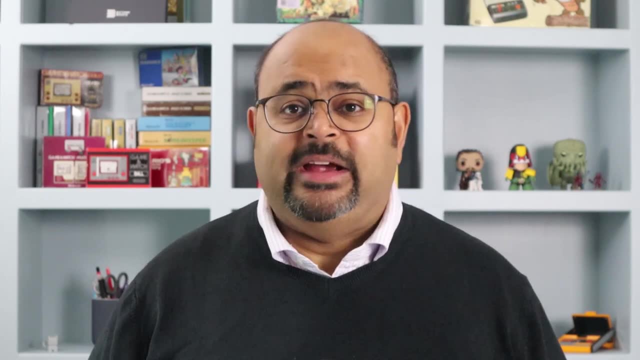 Sitting hand in hand with meaningful decisions are multiple paths to victory. All games allow for some form of progression, but a good game should be able to allow you to have multiple ways to progress. Is the aim for you to concentrate on buying development cards in this particular game of games? 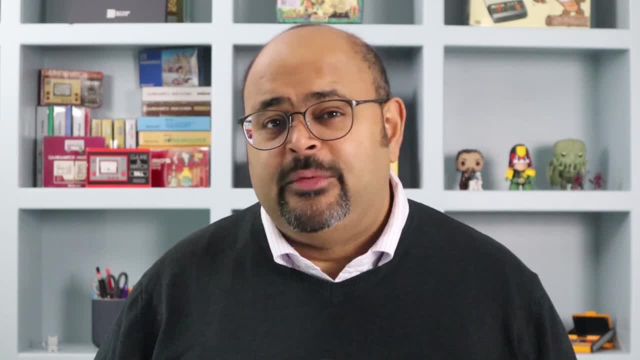 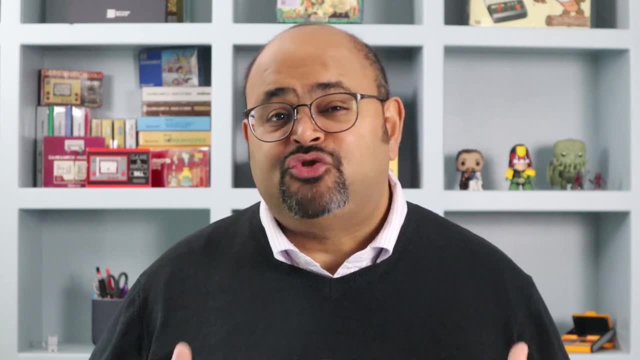 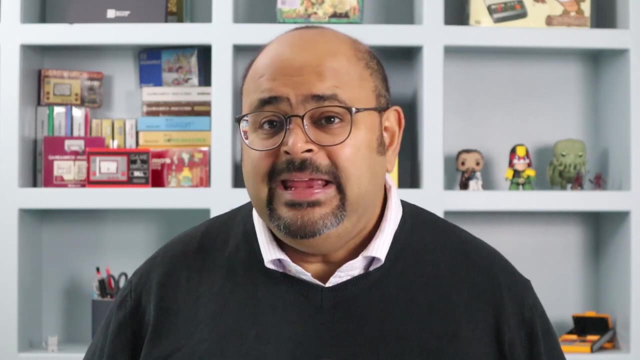 Or is it to build roads and link up different parts of the board? These decisions are, of course, meaningful in their own right, but together they form part of a strategy of play, Any one of which could lead you to win the game overall, And it's a strategy that you may need to change partway through the game, depending on what happens. A good game should enable you to do that. A game with multiple paths to victory definitely makes the game more replayable. Potentially, it also allows for different styles of play and therefore different styles of player. A game that eliminates luck completely allows for no variance in play, and that means a good player will always beat a bad player. 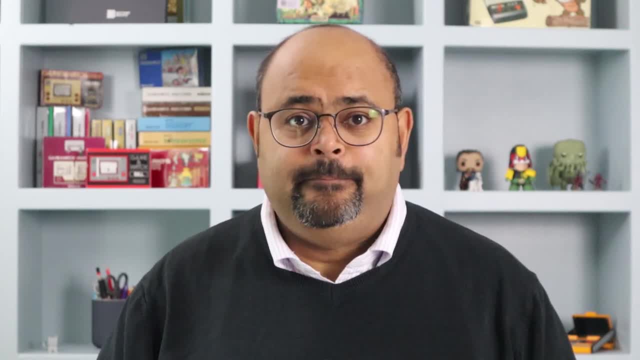 For me, games like chess fall into this category. Conversely, if you remove all the skill out of a game, well then there's no such thing as a good player. In fact, there's no game. You may as well just be rolling dice to see who gets the highest number. 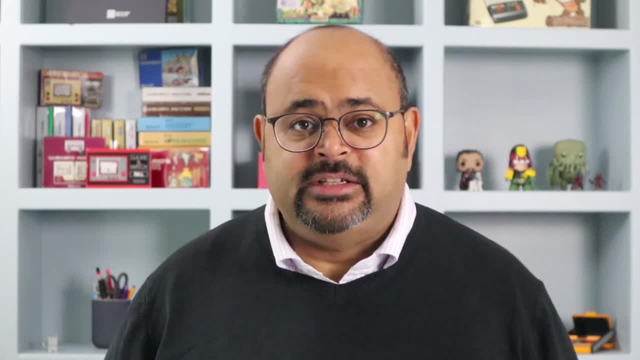 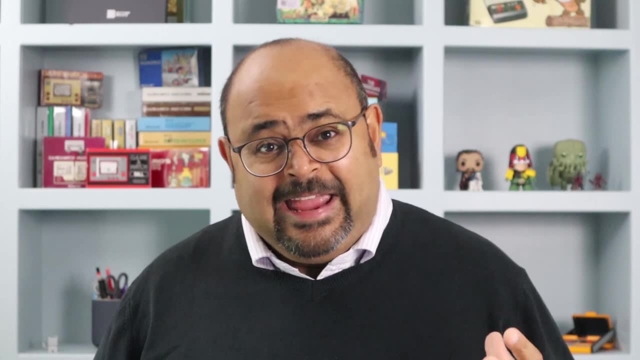 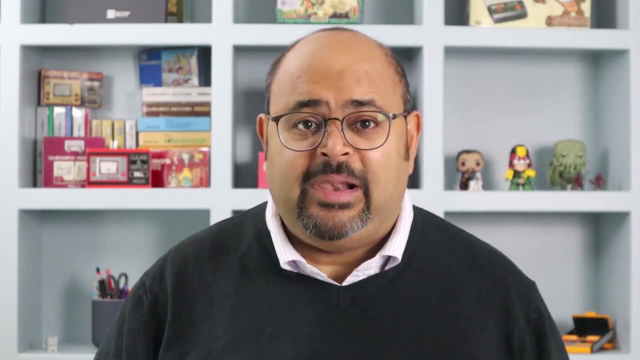 A good game should enable luck to play a part in adding variance, but it shouldn't be solely responsible for who dominates in that game. Then again, a game should have enough skill to enable those meaningful decisions that we talked about earlier to be made often enough to affect play. But not so often that it leads to players spending all of their time working out what to do next- That so-called analysis paralysis. Getting the balance of skill and luck is really important and actually really difficult to do. A good game gets that just right. 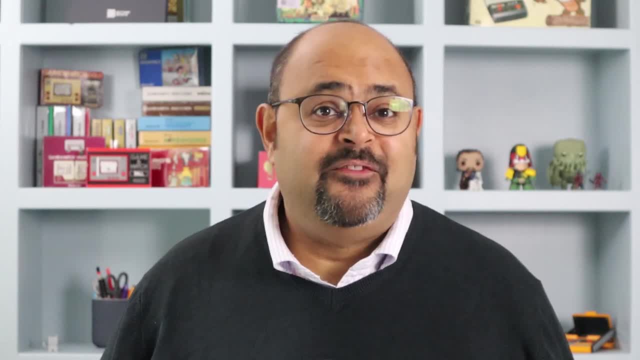 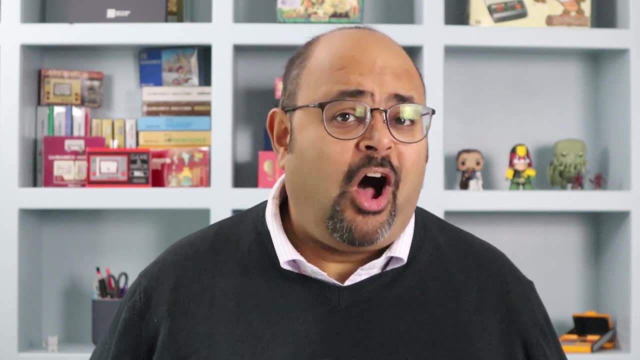 The analysis paralysis comment leads me comfortably to my fourth point, which was minimal downtime. Now, there's not much to say here other than, by definition, a game can't be very good if you spend all of your time not actually playing it. 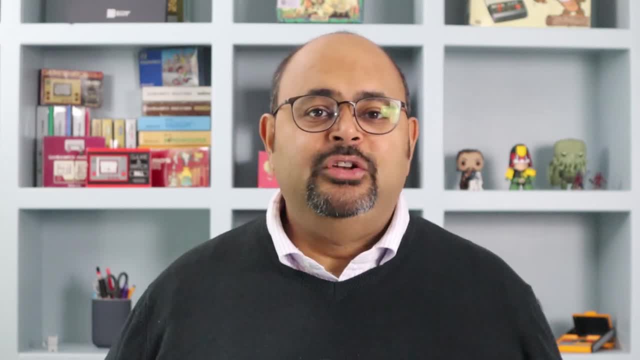 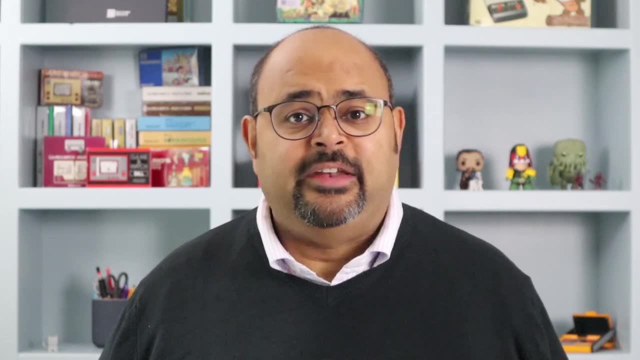 You're either waiting to do something or waiting for someone else to do something. A good game should have short turns with a limited number of actions per turn. I think reference card explaining those actions are usually a very good idea and help with the flow of the game. 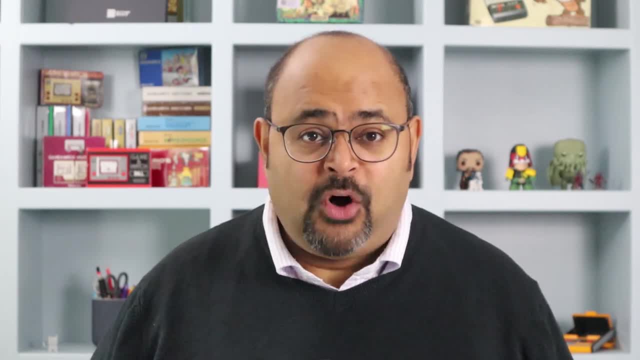 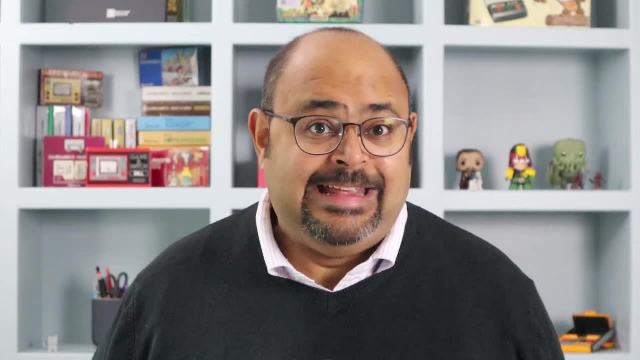 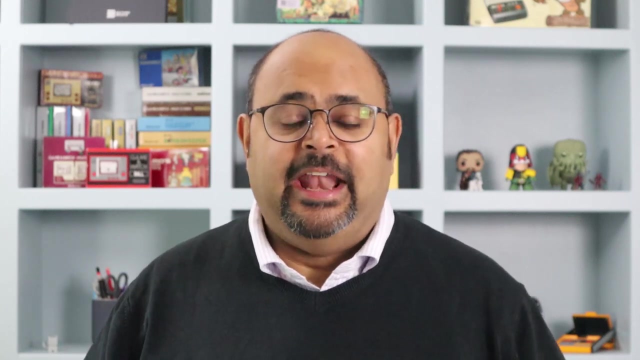 And there's one other final point here: An obvious way to keep players involved in the game is not to eliminate them. So in my book, a good game does not use the player elimination mechanic either. And that leads me to my last point, which is clear iconography and unambiguous text. 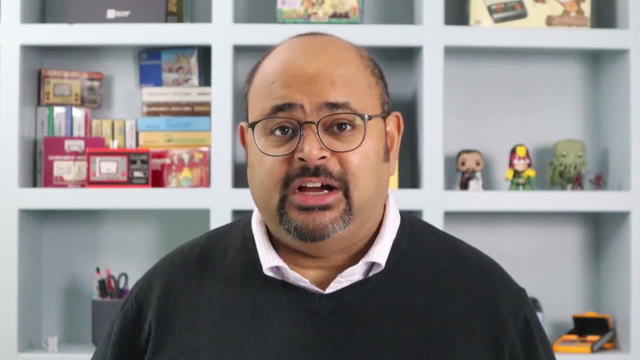 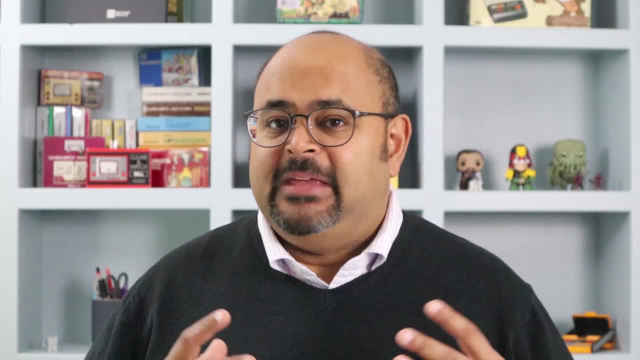 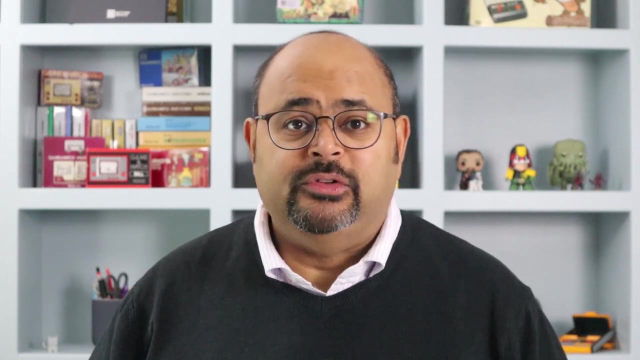 Now, this doesn't mean that all games should have really high production values and expensive playing pieces. It just means that all player pieces- cards, tokens, etc. should be clear and easy to read And they should relate directly to what's described in the rules. 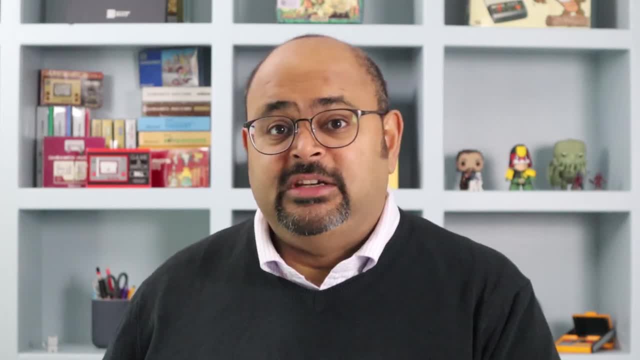 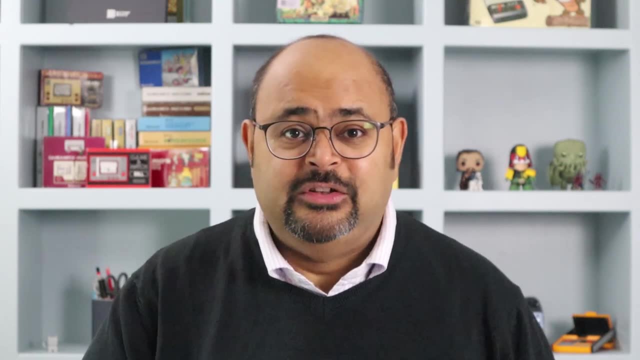 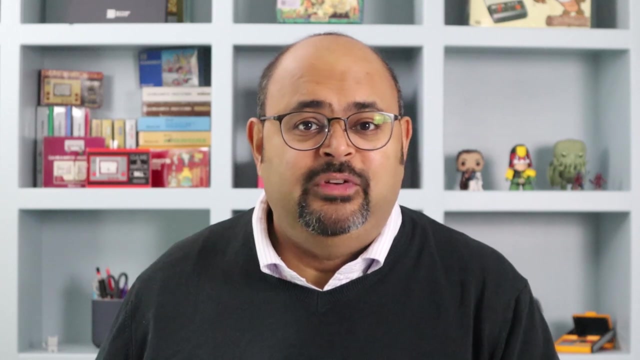 Yellow tokens should be yellow And not a color that could be interpreted as blue or yellow or green. Victory point tracks should be wide enough to actually hold victory point tokens on them And if this is a war game that I'm playing, the playing pieces should reflect pictured troops or fighting units rather than having vague round circles on them. 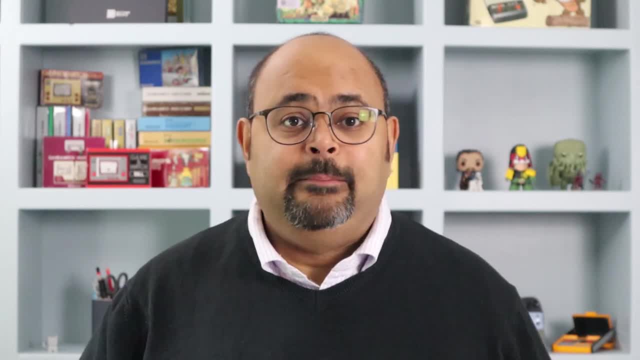 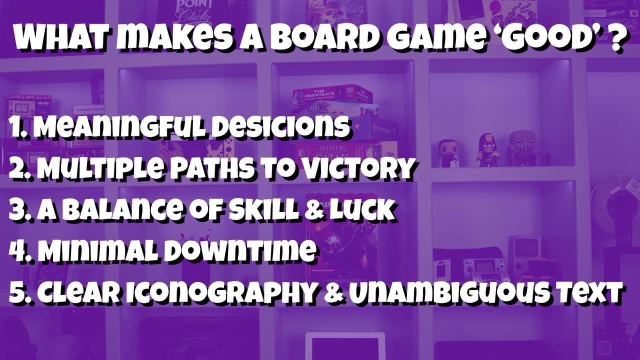 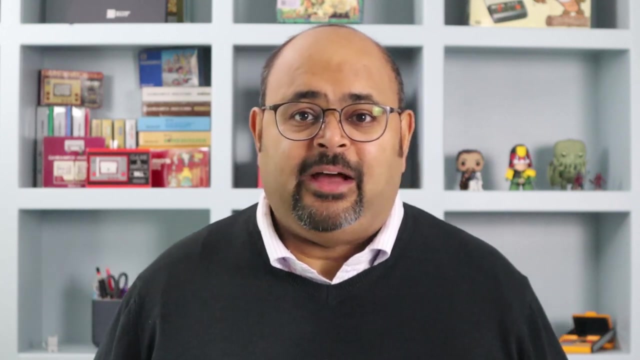 A good game should have components that make playing the game easier and not harder. So that's my list of five. Now, one thing I didn't include was theme, And I did think carefully about this, but I realized that actually a lot of games, at their core, could be reskinned, and often are. 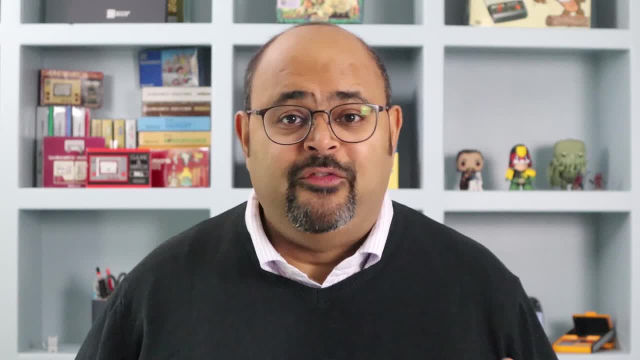 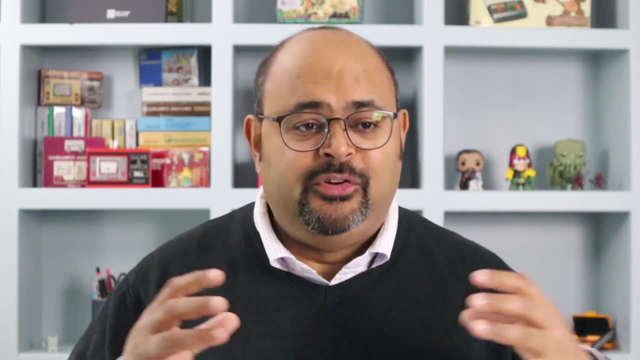 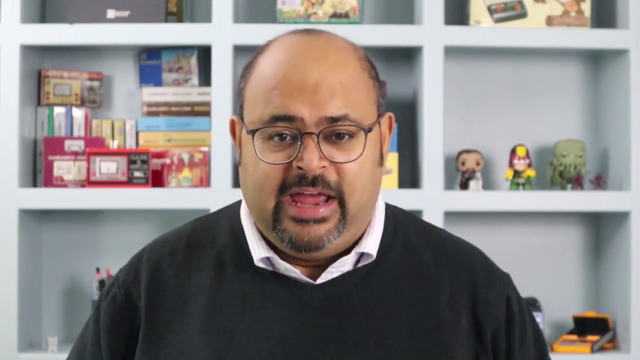 Things like Ticket to Ride, even Monopoly- you can skin over and over again. What may have been important is perhaps the context. If you're playing a game about building railways- going back to the Ticket to Ride example, then I'm not really sure having a war game mechanic where you take over stations would keep in the theme of that game and in the context of that game. 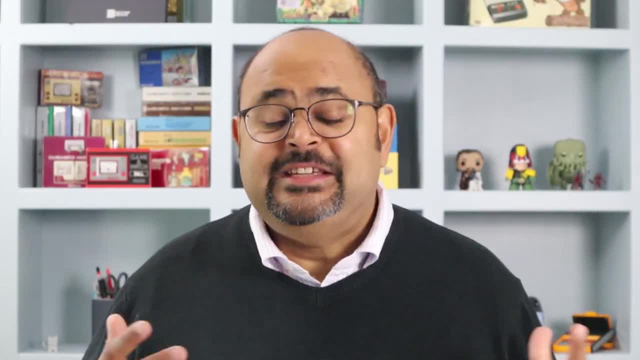 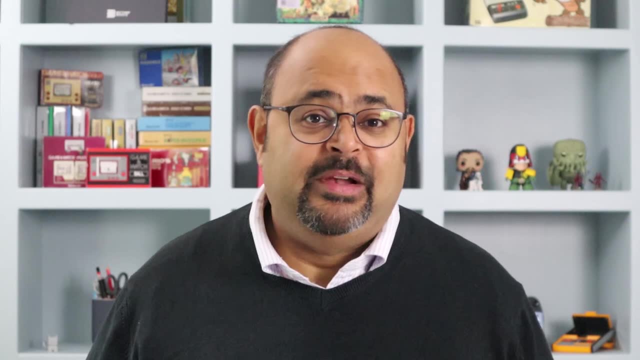 Possibly I could have included that, But as always, this is my own take on what makes a game good. Yours might differ, And if it does, why don't you share your thoughts in the comments below? I'd love to read them. 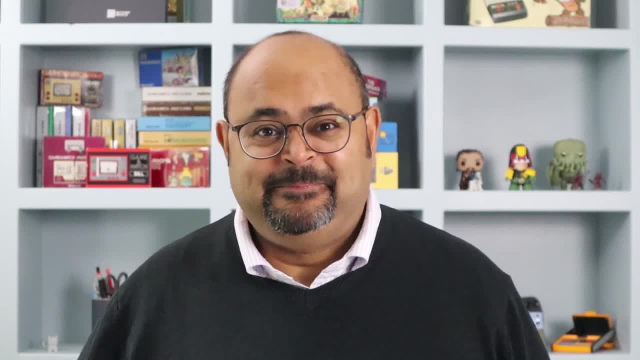 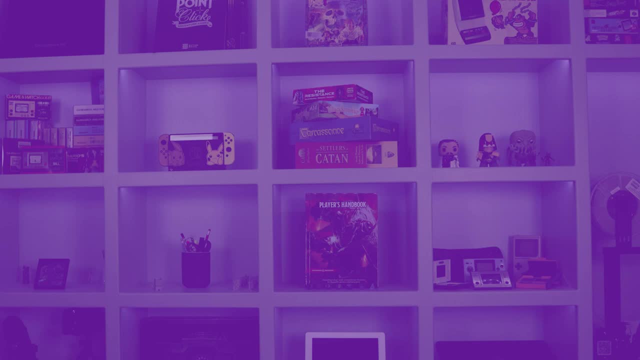 For now, though, and until next time, take care. Thanks for watching.